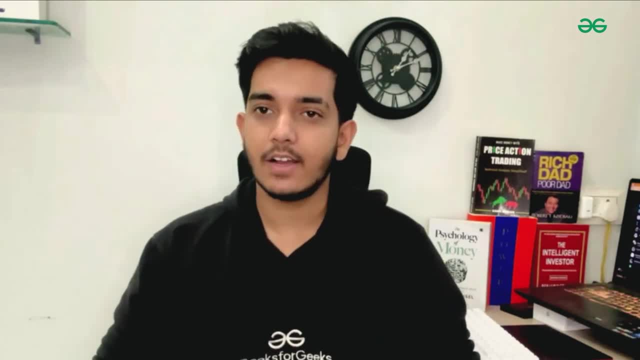 So in this video we walk through seven fundamental JavaScript concepts with easy to understand examples so that any beginner can grasp easily. So the first concept is scope. Scope defines where variable and functions are accessible within your code. Think of it as a range where you can use it. So here is an example: in this code: X can be. 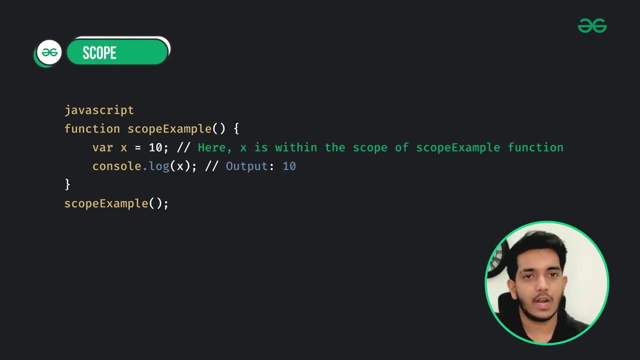 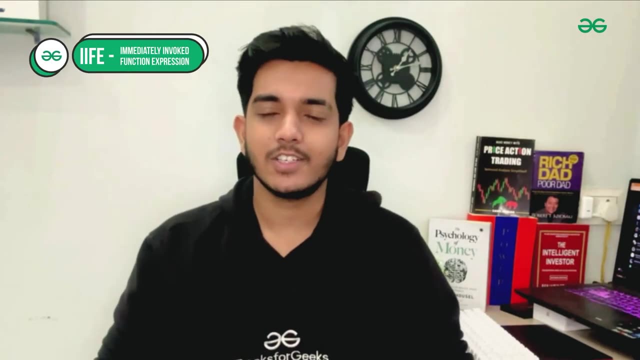 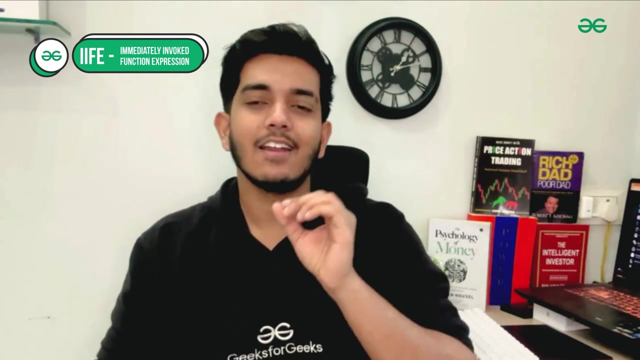 accessed within the function scope, example. If you try to access it outside, you will get an error. Number two: IIFE immediately invoked function expression. So this word might sound complex, but it's essentially a function That runs as soon as it's defined. So it's useful for creating a private space for variables. 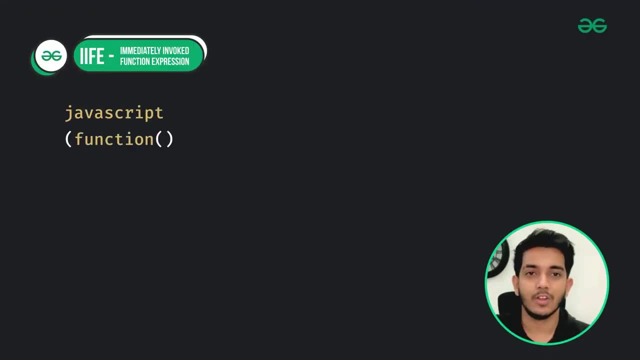 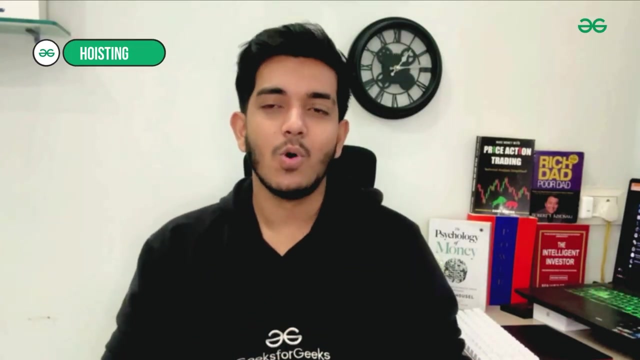 So let's see it with the help of this example. So here you can see that X is scope inside IIFE and can be accessed from outside, So helping us to keep our code tidy and avoiding the conflicts. And the third concept is hoisting. So hoisting is JavaScript's behavior of moving variable. 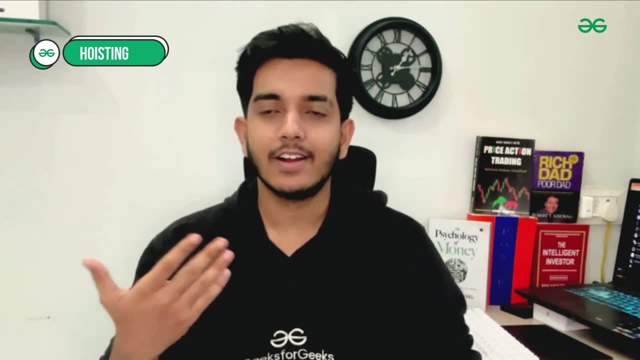 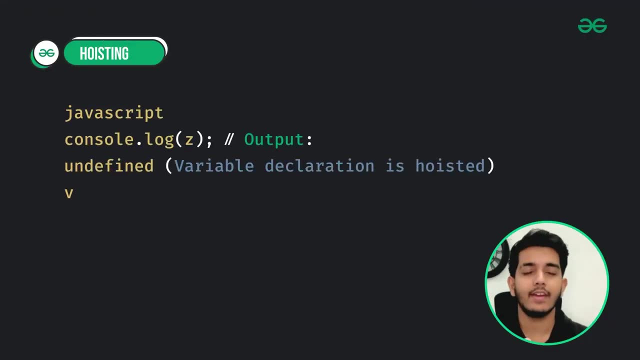 and function declarations to the top of the code, their containing scope during compilation. So let's illustrate to the end of this example. So here you can see that even though we are trying to log Z before the declaration, but JavaScript moves the declaration to the top. 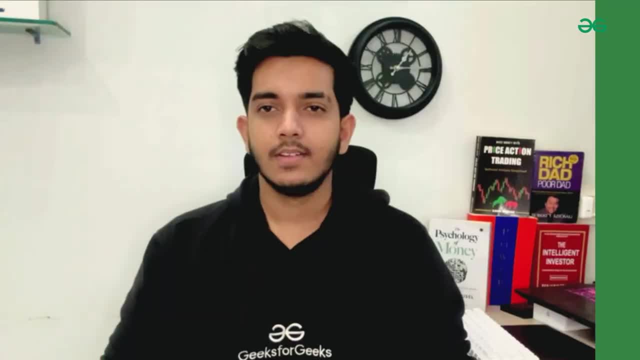 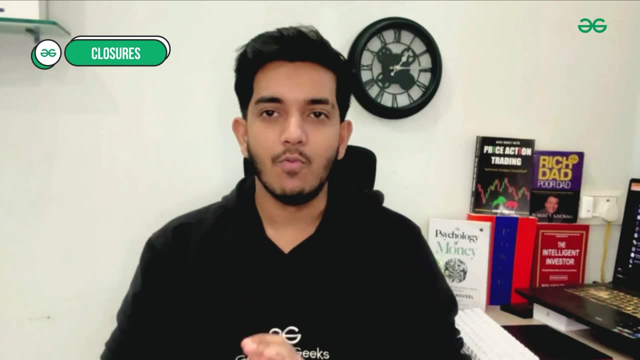 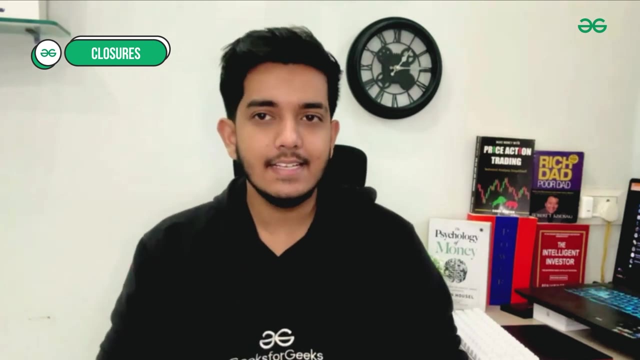 giving us undefined instead of the error. The fourth concept is closures. So closures allow functions to remember the variables from the scope and when they were created, Even if that scope has finished executing. this might sound abstract, but it's easier with an example. 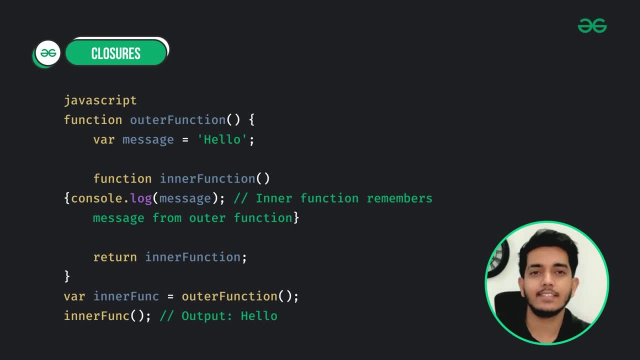 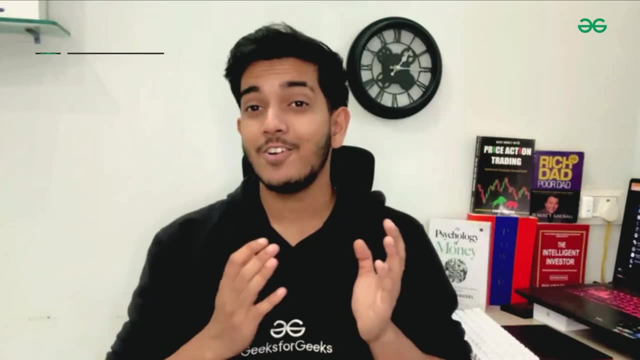 So in this example you can see that inner function still has access to the message variable from outer function even after outer function has finished executing Number five: callbacks. So callbacks are functions passed as arguments to the other functions to be executed later. 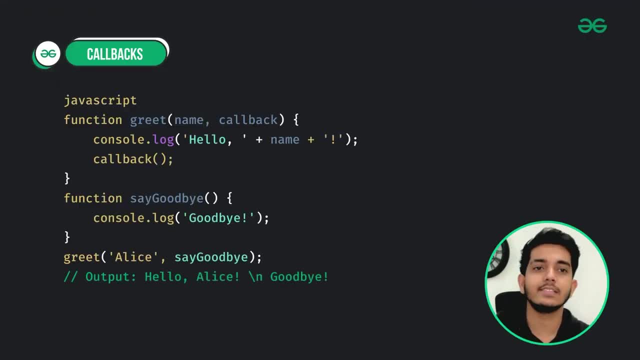 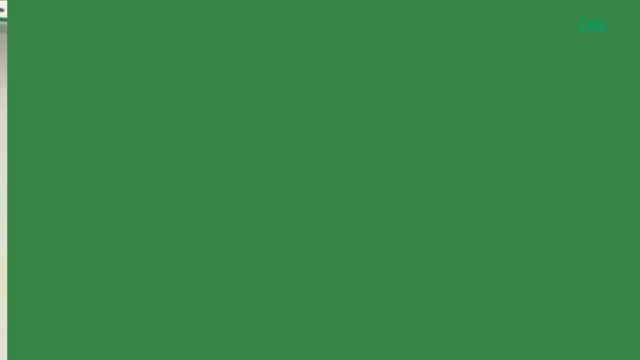 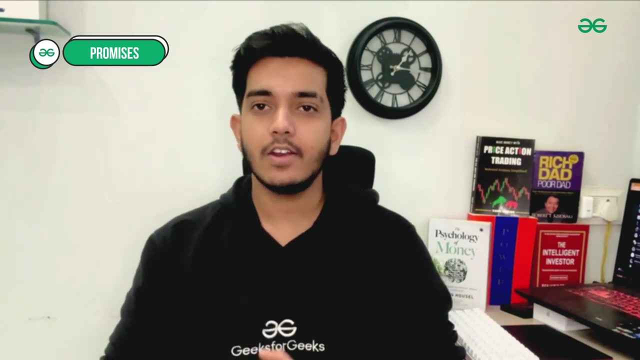 So let's see how it works. So here you can see that say goodbye is a callback function passed to the treat Which gets executed after reading Alice Number six: promises. So promises represent the result of an asynchronous function. They are used to handle asynchronous operations.